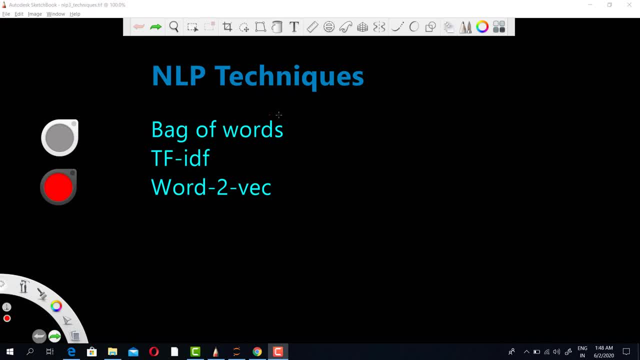 NLP techniques, And we have three kinds of NLP techniques. One is the bag of words, Another one is the TF-IDF and then Word2Vec. So in this video we are going to learn about these two techniques- bag of words and TF-IDF- because that is what we are going to use in our modeling part. 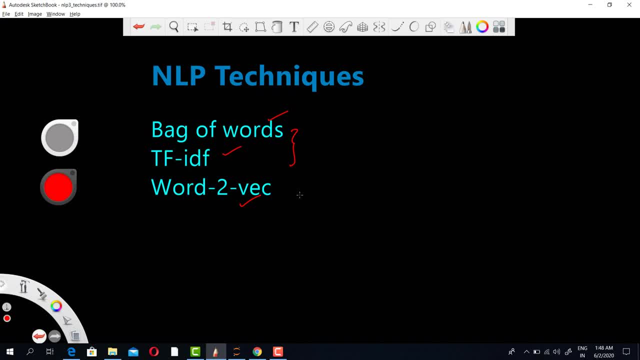 as part of this series And Word2Vec. I'll create another video so that you can understand how Word2Vec works. So let's come back to the bag of words. So bag of words is a very simple process where, let's say, you have two sentences, Sentence one says: 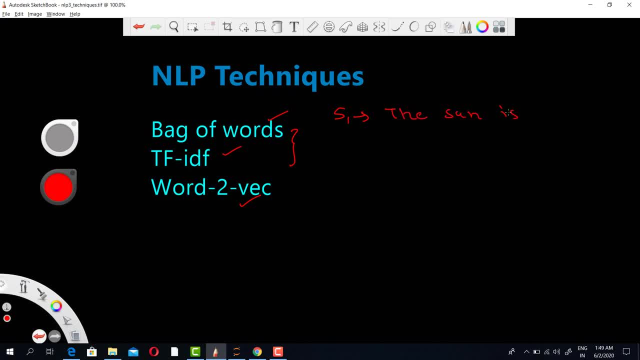 the sun is shining And sentence two says the rain is pouring. Now you can see that we have some unique words and the sun is shining. four, five and six. Here you can see that we have six unique words right, So we will use the bag of words. and the sentence two says the rain is pouring And sentence two says 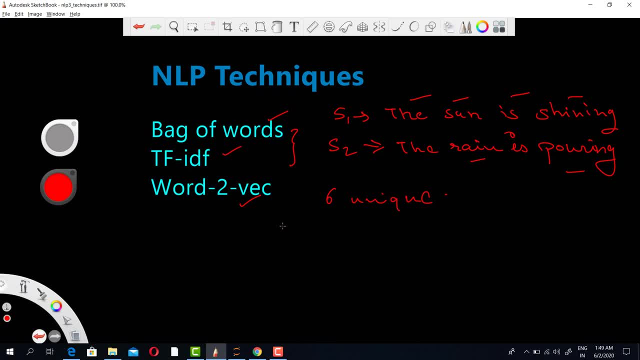 the rain is pouring And Duchamp says, finally, the rain is pouring. So now, with, according to the mx meaning, it is called the bag of words. But we will go further and see what happens if we recommend the bag of words, because actually this isn't a bag of words. let me show it to you Now, here. 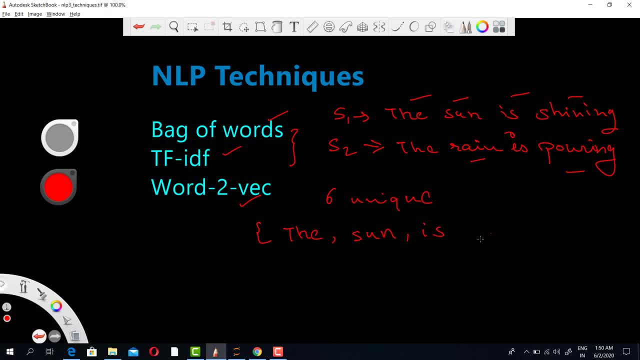 we have two different words in our model, So the word bag of words in draws out a complete sentence from the bag of words. The window which is showing us the income, revenue and abges круal of this month is actually the word which outputed from the sales transaction in. 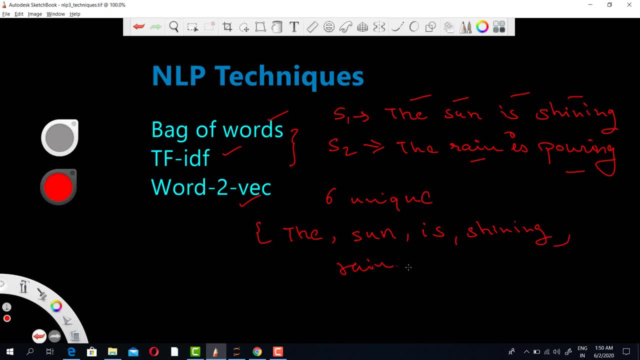 other wordsriıp olarak a lot of money. So once again, days upon days or even many more years, they accordingly say: the back of words are kind of like same, something different which they don't buy, or connect everything When making almost any kind of tag. 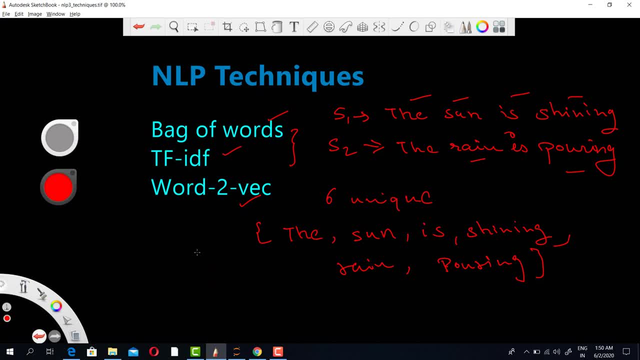 for example, there are all kinds of lecturer who talk about price and helmet and all that sort of. create a dictionary where we will have the values also. da is coming two times, sun is coming. once is coming two times. then we have shining one, rain one and pouring one. so how? 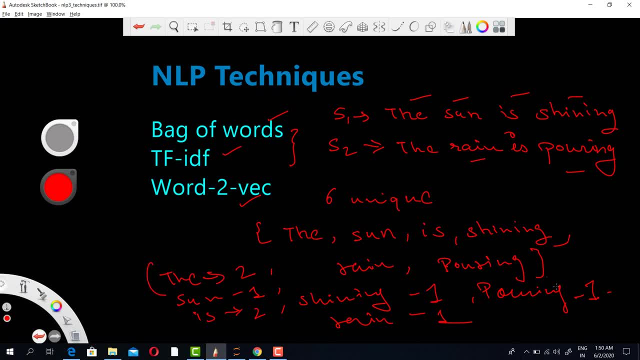 bag of word works is we replace these words in the data with the frequency. so that is why it is also called as count vectorizer in a scale and because it works on the frequency of the words. so let's see one example of this bag of words. so if you want to import the bag of words, you will have 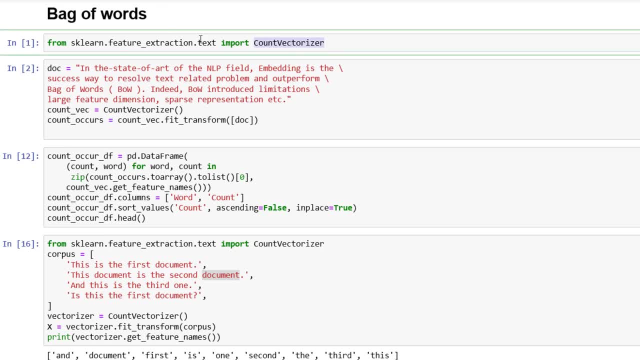 to import this count vectorizer from a scale and feature extraction dot text and this module will give you the count vectorizer. and now I have some sample sentences here. so we have in the state of art NLP field. embedding is the success way to the resolve text related problems and outperform bag of words and all these words. 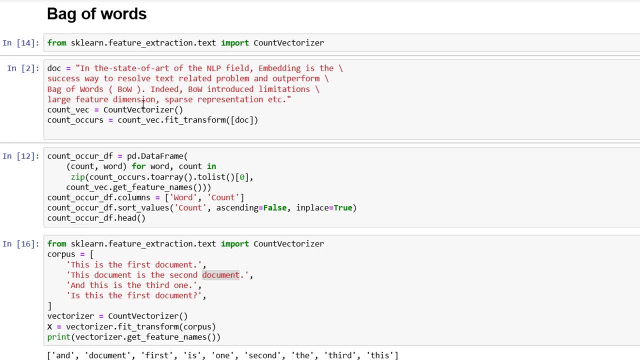 are there. now what I'm gonna do is I'm gonna import this count vectorizer in an object which is count wet here and I will use this count wet to fit and transform on this complete document. so what is this fit and transform? I will explain in a while. 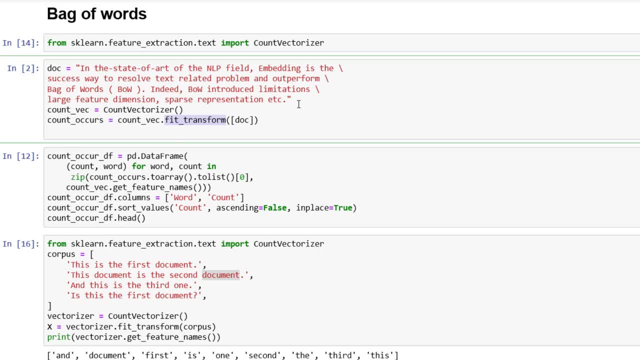 but just imagine for a second. I am going to convert this whole text into its frequency, which I have shown in the example earlier, right? so I will just run the cell and now you will see that this count underscore occurs will hold the frequency and this count vec, which is here the 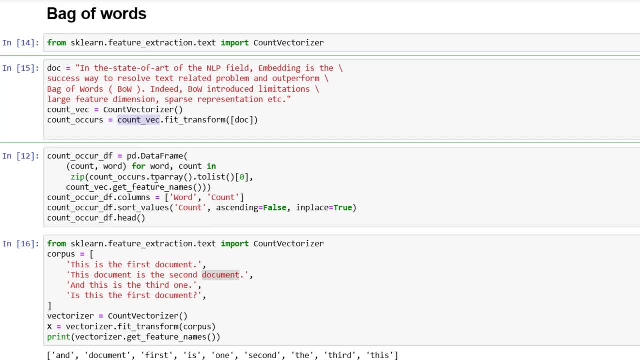 object will hold the features, the words, in distinct words. all right, so what you can see here is I have created a data frame from these two things: one is the frequency and another which is the words, unique words, which are the features in count vec. so, and I have given the columns word and count and 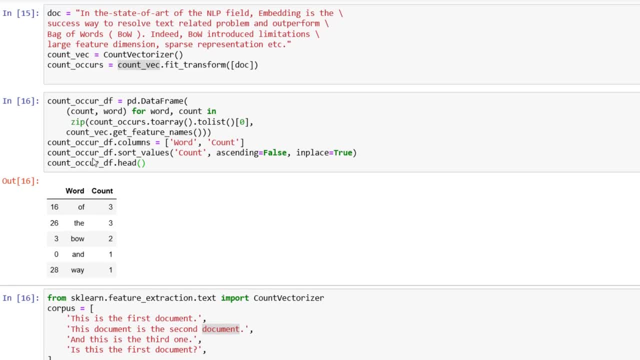 if I run this cell, you will see that all these words here are. I have printed a first few words using head right and you will see the frequency. so off is coming three times, as you can see: once here, then once here right and once here. similarly, if you see other words like b o w, bow, it is coming once. 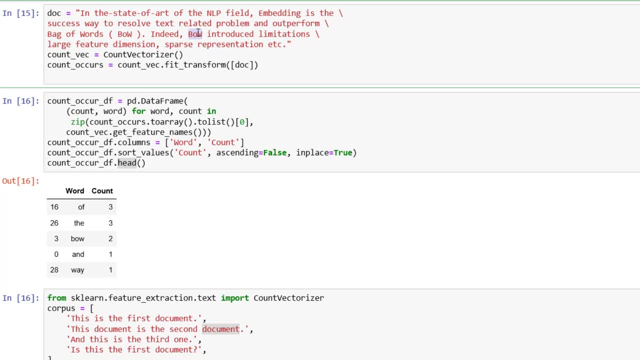 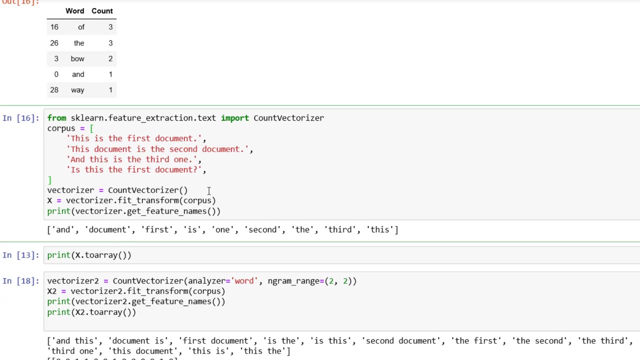 here, and then it is coming once here. so this is how count vectorizer works. it has converted the words into its frequencies. so let us see another example. like I have declared a corpus here with different, different sentences and I have used count vectorizer in an object vectorizer and again I am doing fit, underscore, transform on this corpus, and then you 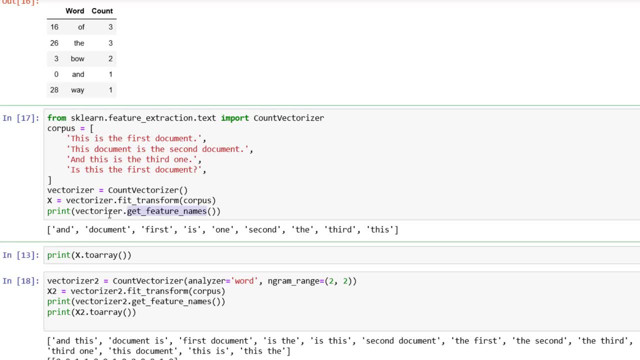 can see. you can call this, get feature names with this object and you will get all the words that are there in this corpus. as you can see, all the words are there in one list. let us see the count, the frequency, which is we have stored in this X part here. right, I am converting this X to array. 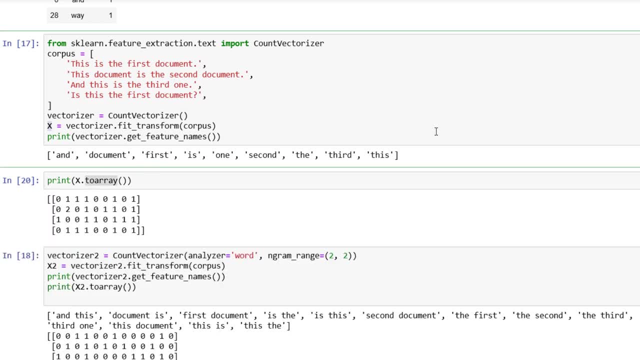 here, and and you can see that all these words have corresponding frequencies for each sentence. for example, and is occurring zero times in first sentence, right, that's why it is zero here. document is occurring once, you can see this, so that's why it is one. similarly, if you see the second sentence, 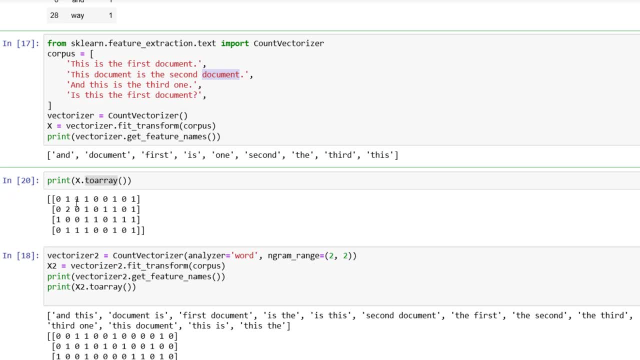 you will see that document is coming twice. that's how it is replaced with two here. similarly, if you see this second sentence and the third word, which is first here, because these are the features, and features will remain in this shape and only the numbers will change in the 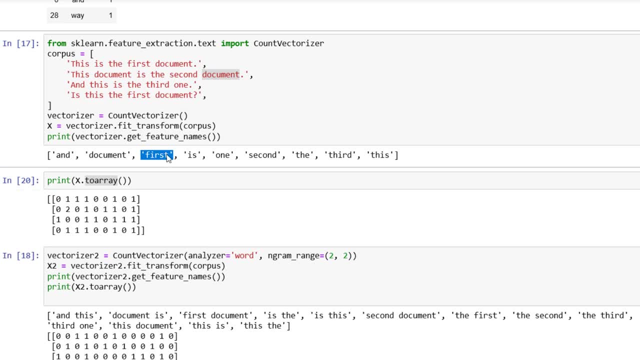 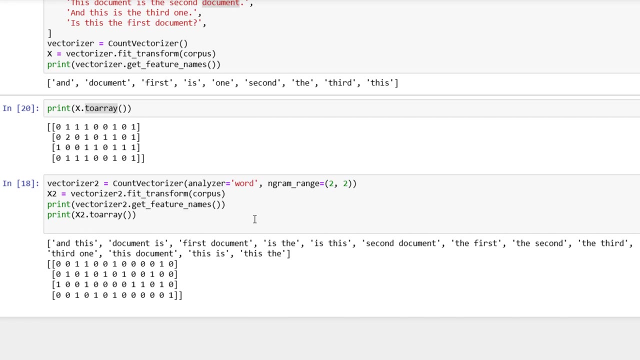 sentences, all right. so if this word is not present in that particular sentence, it will be zero there, all right, so that's that's how simple the bag of words it is. so again, there is one more example here. so you can also pass n grams to the bag of words. so what is going on here is I am giving n gram. 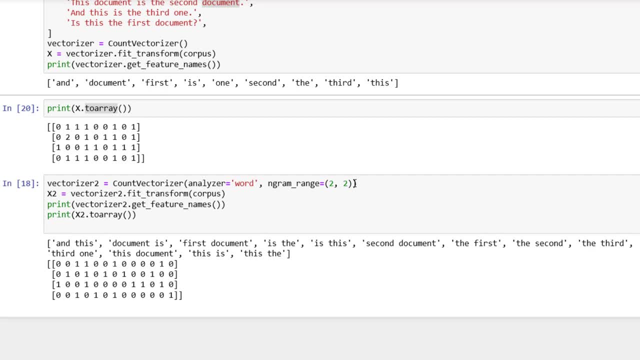 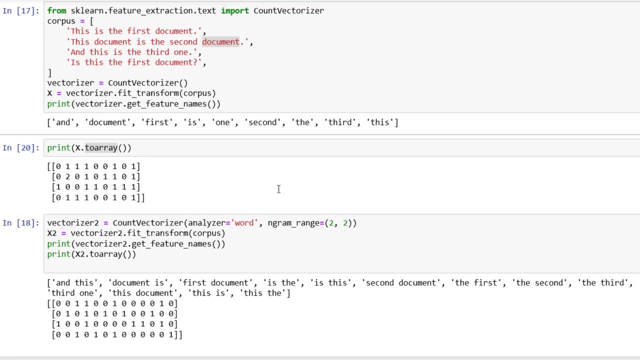 range 2 comma 2, which means that it will only take words with two words. it will only consider two words together as one word. for example, all these words, if you see here, have been collaborated into two words. for example, and this is now one word, this is is now one word. 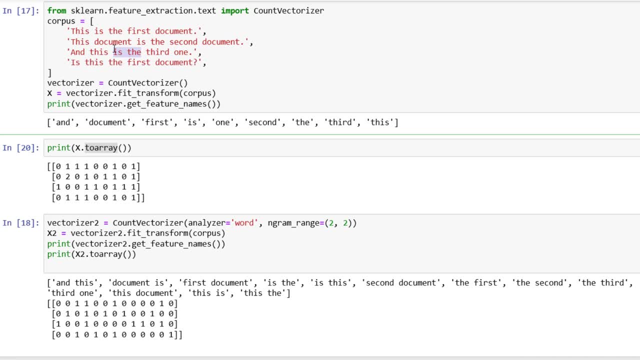 is, the is now one word. so these kind of things is important. when you see, in life we have, for example, a company name: Tata consultancy services. now, Tata consultancy services. these are three unique words, but individually they don't hold any value. right, they don't represent the organization, but together, 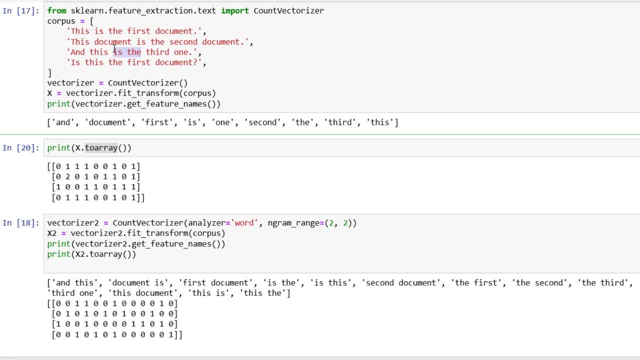 these three words come together to represent an organization. another example is Birla soft. Birla, a different token, a different word, soft is a different word, different token, and both have different meanings, right, but together they form a unique entity. that's where n grams comes into play. so if I give the range n, 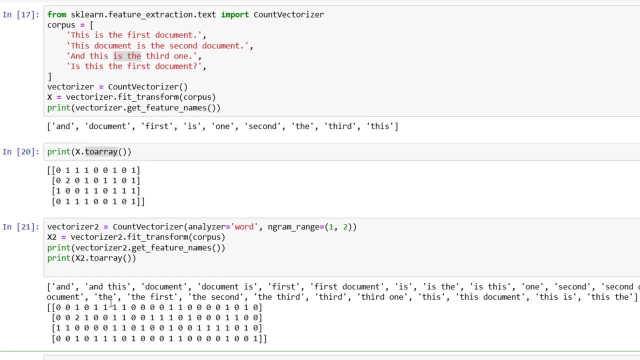 grams range from one to two. here you will see that my single words and the double words are both are included. so you will see that is is the right document. document is all these things. range becomes one to two. similarly, if I give range three, here you will see that my feature size is getting increasing again. and 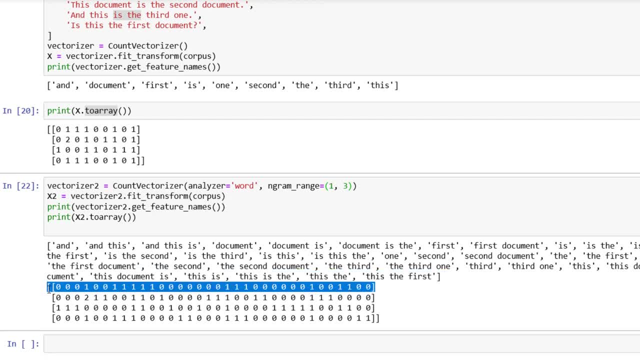 again, because it will take all the permutation combination from range one to three, right in the series. so you will see that and this and this is so that simple is the bag of words to understand, but it has its own limitation. here you can see that the construction of sentence doesn't play a. 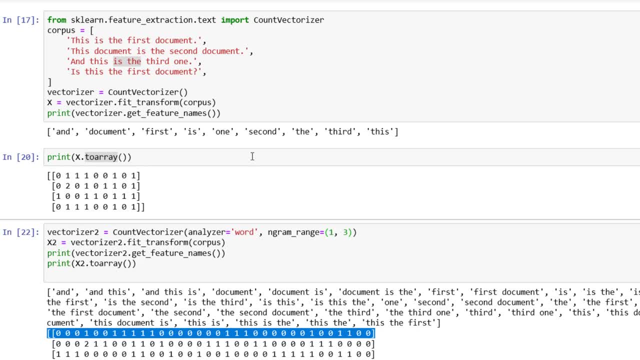 it doesn't play an important role, right? it only works with the unique words it doesn't have to take. it doesn't take care of the construction of the sentence or the grammatical expression of the sentence, and a lot of Limitations are there. that's why we now come to the point where we 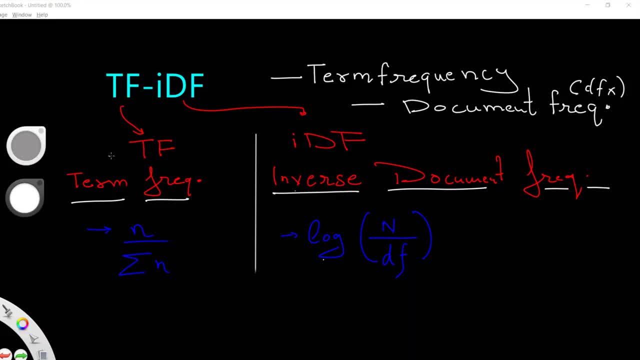 use TF idf, so let's move on to the TF idf. so in TF idf we have two things: TF and idf. in NLP we have a few items from the builder to make YOU zeggen and IDF. in NLP we have a few things were let's see아. 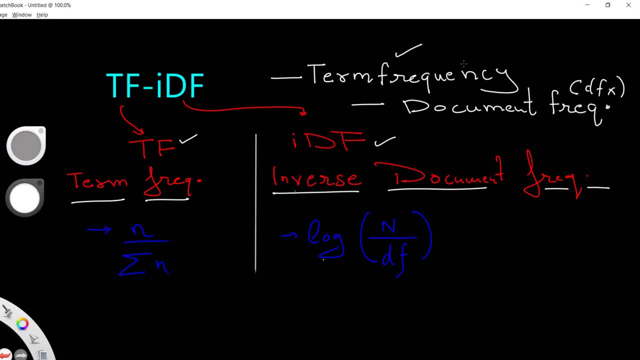 وっと, we have few terms like this term: frequency, document frequency and inverse document frequency. so what is term frequency? term frequency is the, let's say, for term frequency of word x is the count of word x in a document. count of word x in a document divided by the total number. 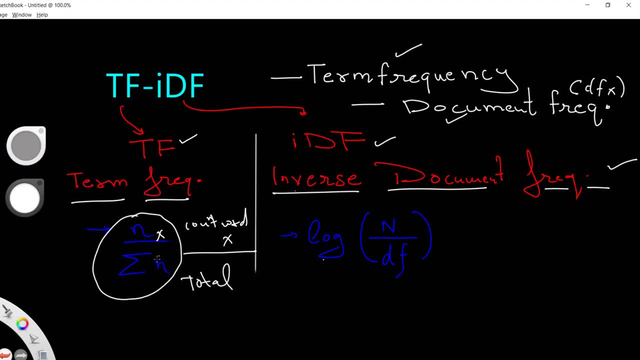 of words. all right, this is what this formula is saying. now, what is the document frequency? so document frequency is the total number of documents that contains the word x. that is why it is denoted by df x. so x is the word okay, and the total number of documents that hold x. now, 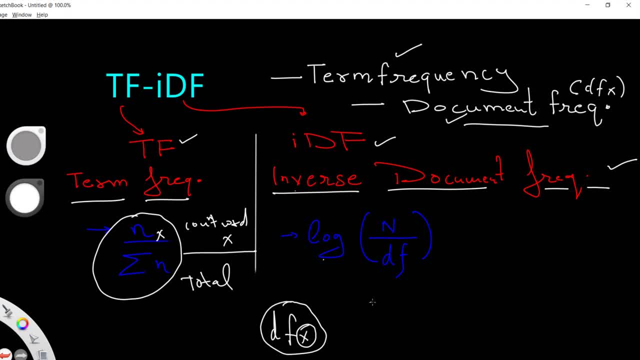 inverse document frequency is similar to document frequency, just that it is the log of the total number of documents divided by the document frequency and the tf idf will come out to be this: this: this tf that we calculate here and idf that will calculate here, multiplication of both term frequency into inverse document frequency. so the whole idea of tf idf. 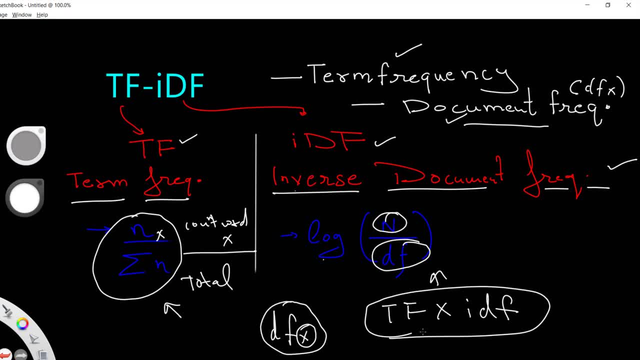 over bag of words or count vectorizer that we have seen earlier is simply that the words that are present in abundance will have higher tf right. their term frequency will be higher, like the is are. these are conjunctions or determiners that is majorly used for the construction of the. 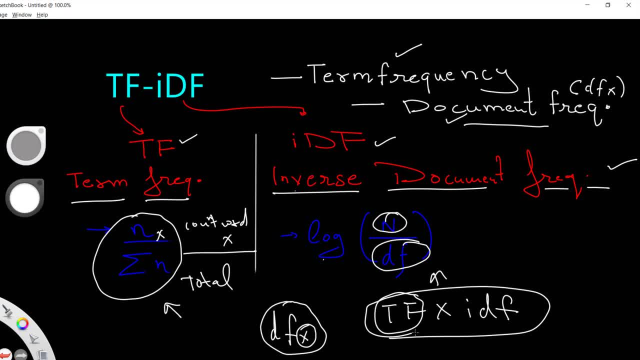 sentence and does not hold any much impact, right any much meaning to the sentence. so that can be normalized. that term frequency can be normalized using idf. so in idf the words that will be in abundance will have lower value. let's see this with an example. so let's say i have two documents. 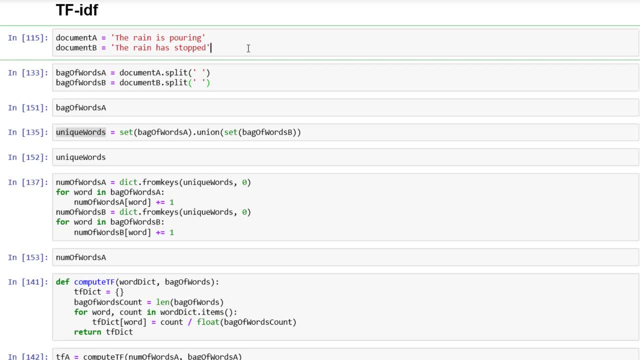 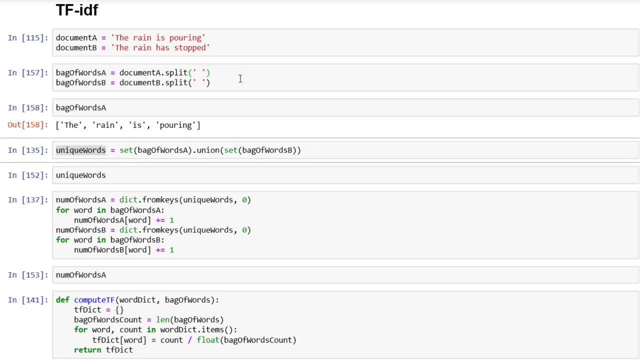 here. document a holds the rain is boring. document b holds the rain has stopped. i will just tokenize those words here and you can see, in bag of words a i have the tokens of this document and in back of words b i have the tokens of document b. so now the unique words will be the union of both, which. 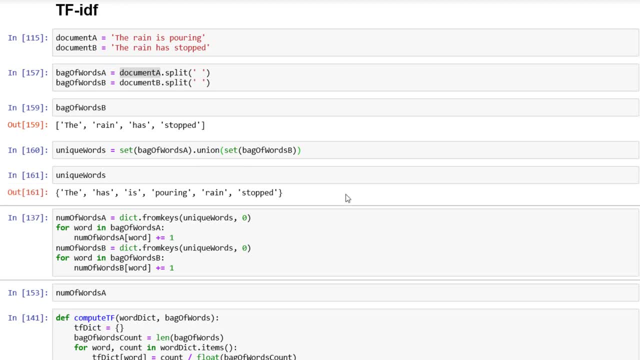 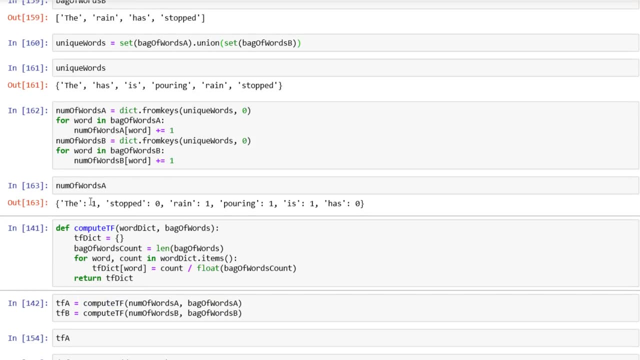 is what i have taken here. right, all the words are there in this unique words. and now what i'm going to do is i'm going to create a dictionary with the words that are present in abundance. so that count of words. so you can see, this is kind of a term frequency where the is coming once in the. 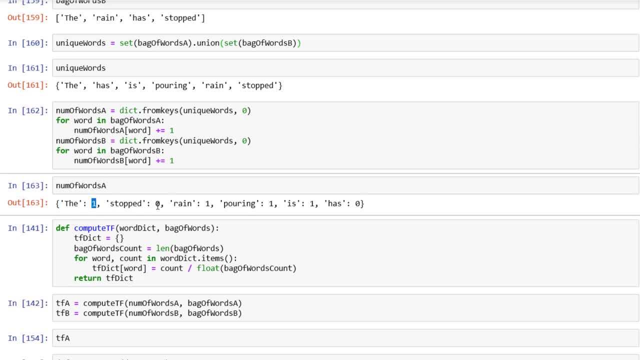 document: document a. so that's why it's one here. stop this coming zero times. it is not present, that's why it's zero, and similarly it will be for b here. so what is happening here? i am just counting the words and creating a dictionary. now my whole idea is: first i need to know the term frequency. 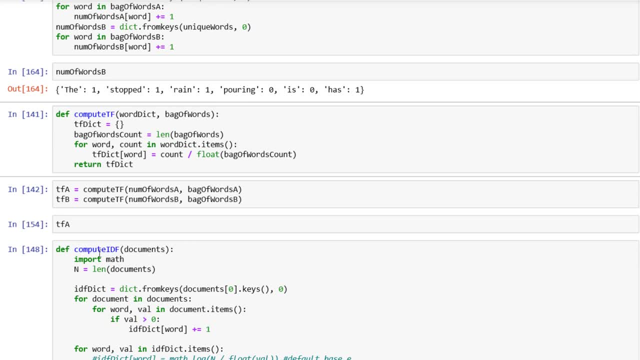 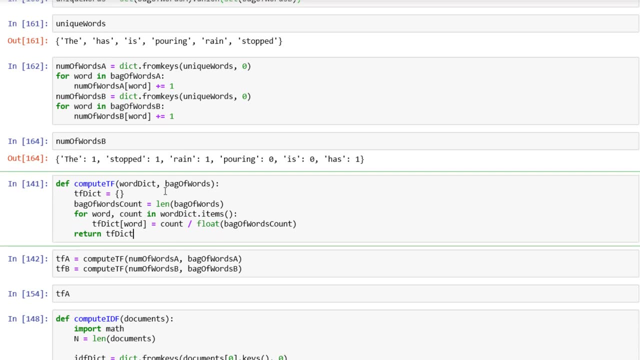 for all the words. then i will calculate the inverse document frequency. once i have both, i will just multiply them. so in term frequency, what i'm going to do i am just simply passing this dictionary and all bag of words. so bag of words simply is all the words right. so what happens in compute tf? 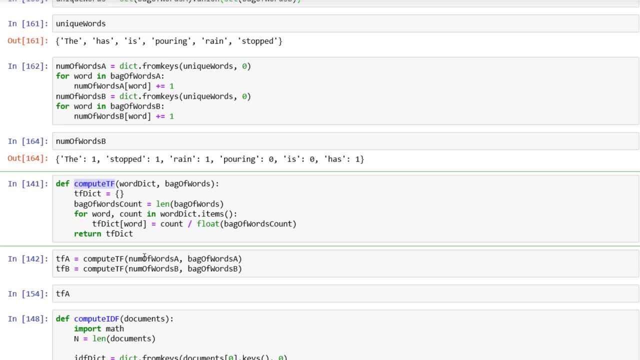 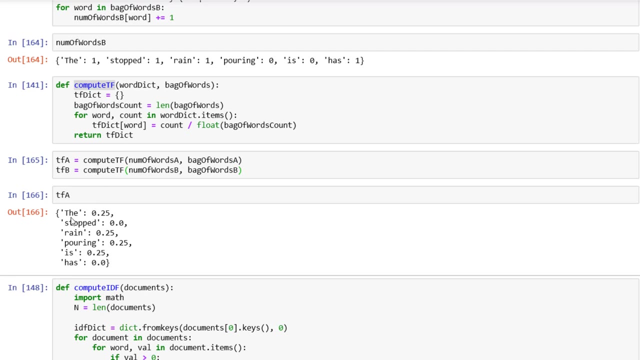 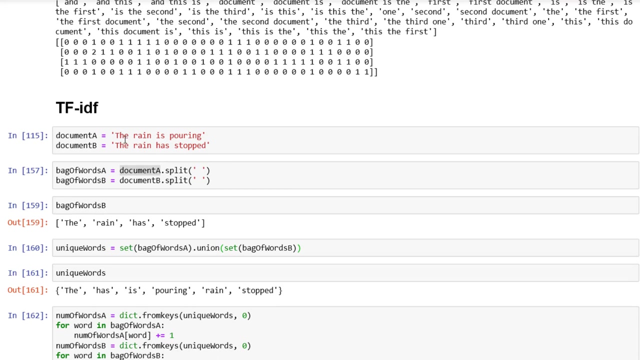 it is just i am counting these words and once i have passed this number of words, this dictionary, and all the words of a, so let's compute this and see that tf of a turn, frequency of a, which is the number of words of the document, a, the is having the term frequency of 0.25, and you can also see. 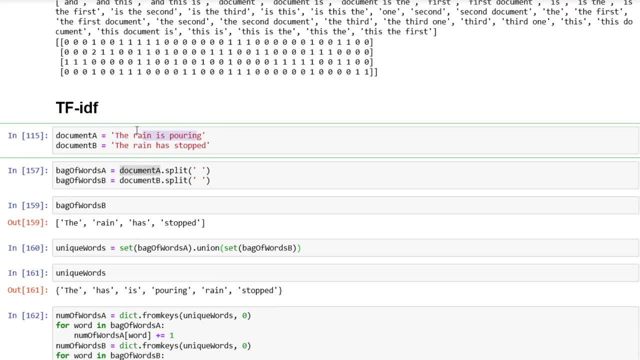 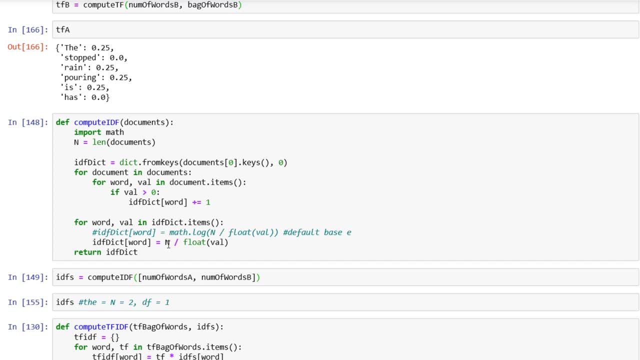 that here the is coming once right and the total number of words are 4. so 1 divided by 4 is 0.25, so nothing much. now what happens in compute idf. it will be the log of, so i will just show it now. 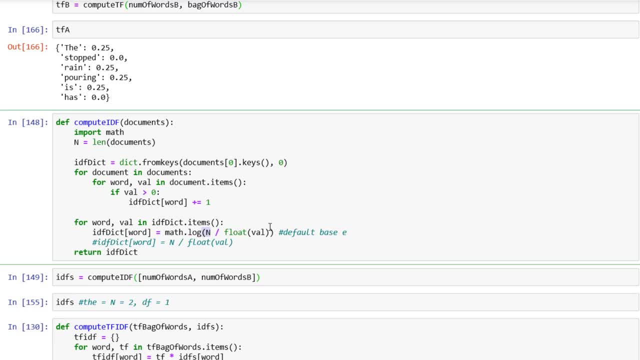 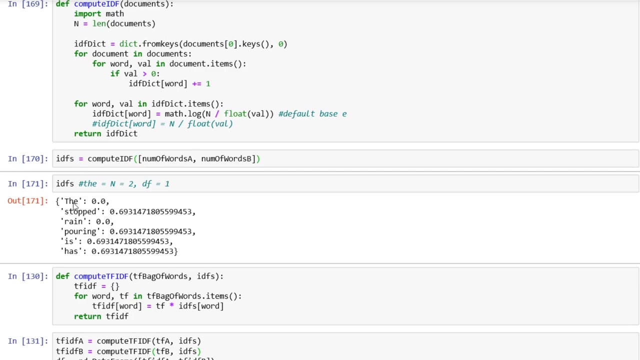 it will be the log of total number, of the total number of documents the word contains, which is what is present in the variable. well, here now i am not going on all this logic. i will quickly show you how the output would be. so if i compute the ids, i will have to pass the same things again and you can see the idf of da is zero and 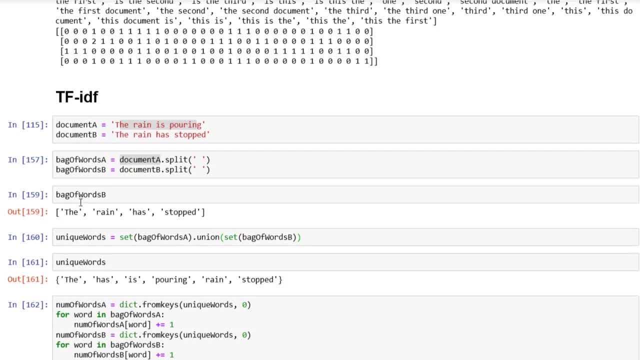 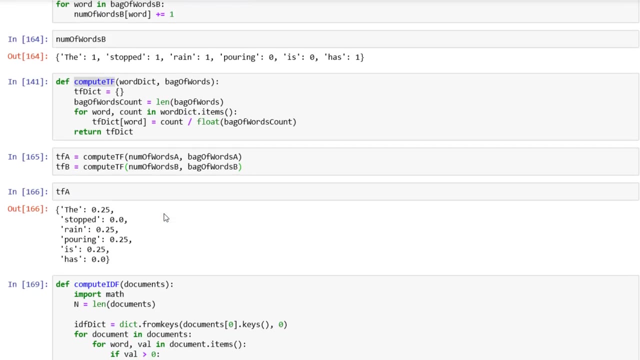 you know that da was coming in both the documents, right, you can see here. da is coming in both the documents, so n is equals to 2, the total number of documents are 2 and document frequency of da will also be 2, right, so 2 divided by 2 is equals to 1 and log of 1 is 0. that's why you can. 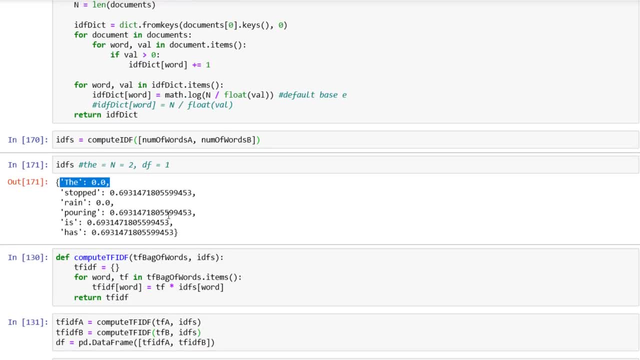 see here, the value of da is 0. so similarly it has gone for all the words and now if i just show you without the log, you will be able to relate it better. now you can see that for da it is without log, it is 1 and with log, log of 1 is 0. similarly for 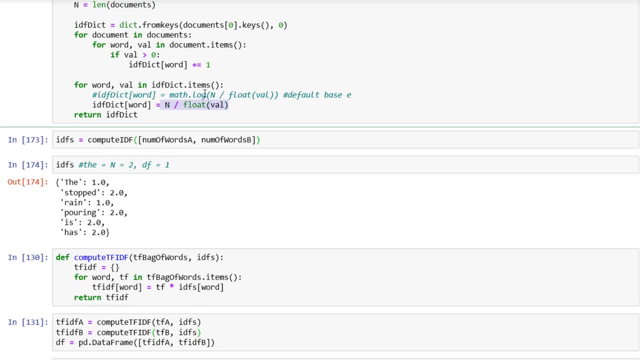 all the words. now, that is what i have done here. i have just removed the log function. so now that i have both term frequency and inverse document frequency, what i am going to do is i am going to compute the tf, idf, which is what i am doing here: i am computing. 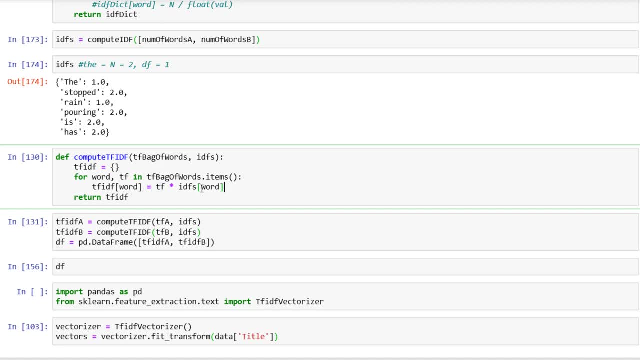 that i am multiplying the tf term frequency into inverse document frequency of that word and similarly i am passing the values here and then when i will call the function and now you can see that term frequency of document a, the frequency of document b and then print the data frame you can. 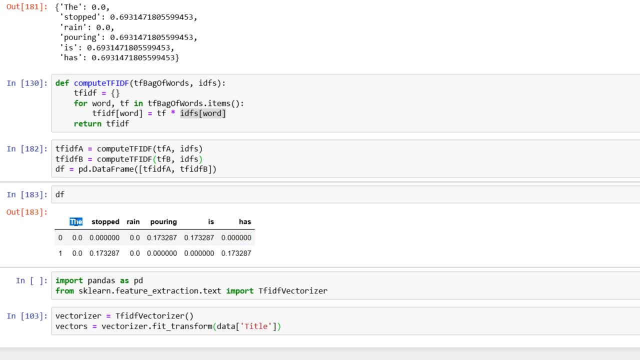 see that my words, like the, which were coming in both the documents, and rain, which are coming in both the documents, their value is now 0, right, and the words, important words like pouring stopped and has, all these words will hold that value, and the foreign ones also, and now this work, they will start. to put into file. you can see that. so this will 100% provide the information that i am using. that is important, but they are not going to get p POR and if you are usingиссcha with pp, it will stops and get. i praise you because i am going to do things like this and this is not going to exist if walsh is coming in. 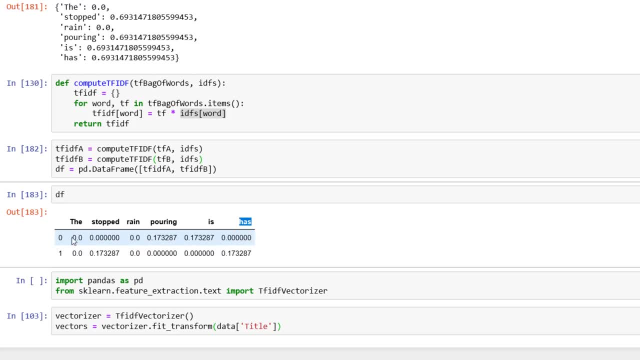 on purpose, automated. and now we have to create ave. so, like showing you what i am going to do, we are going to hold the value. so, just like in document one, the stopped is not present, that's why it is zero. its tf was zero. and in document one, the idf of da was zero. similarly, that's why it is zero, zero, zero. 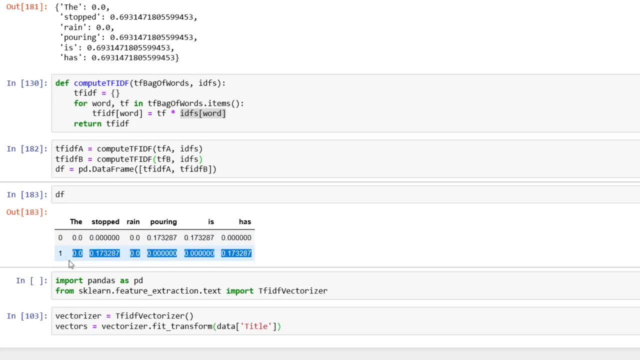 for four words and in again document two. so what happens in tf, idf is simply you give more weightage to those words that are rare. what happens in count, vectorizer or bag of words? there was no such criteria where you will give weightage to the rare words also but the words that are present. 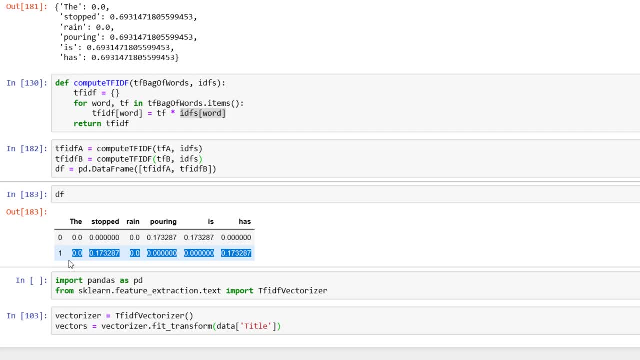 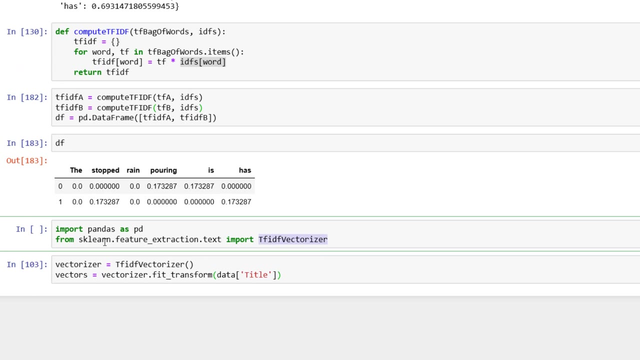 in most abundance will hold the most weightage. so that's why we have gone for the tf idf. and now if you want to apply the tf idf, you just have to use the tf idf vectorizer. so just don't worry about all the code that i have done here, just import the tf idf vectorizer from sklearnfeature. 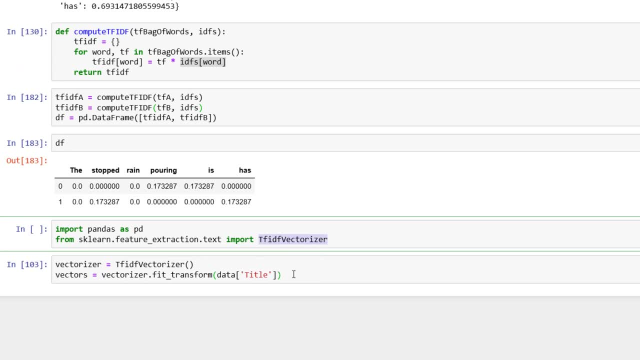 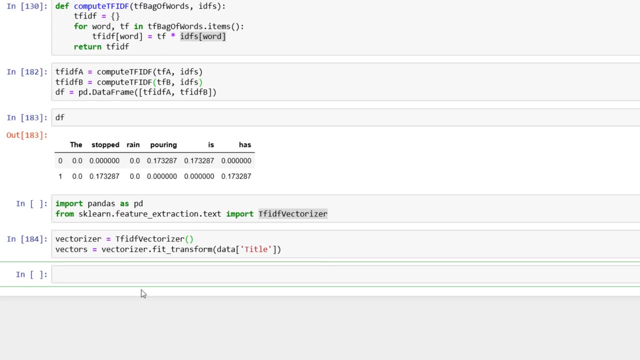 extractiontxt, and then you can apply this on our data, which we have it in the data text. so that's why we have gone for the tf idf. and now, if you want to apply the tf idf, you just have to use the title. all right, and i will run this. and now you can see. 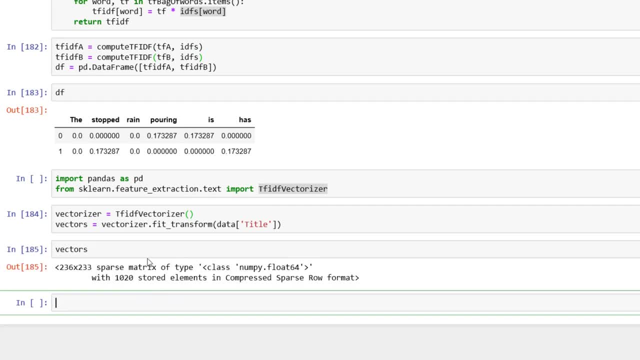 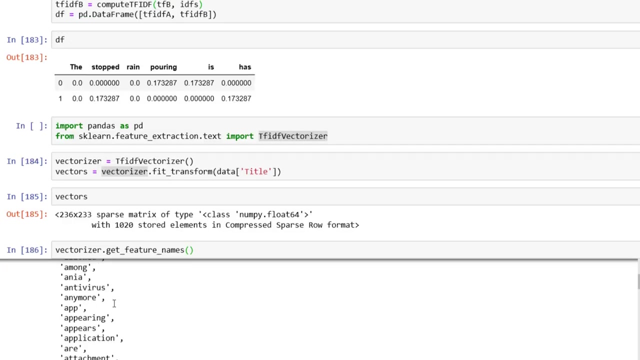 my vectors is a sparse matrix, right, if i? if you just want to quickly see the num, all the words, what you can do is you can use this vectorizer, paste here and then print, get feature underscore names and you will see a list of all the words that are present in the data text. 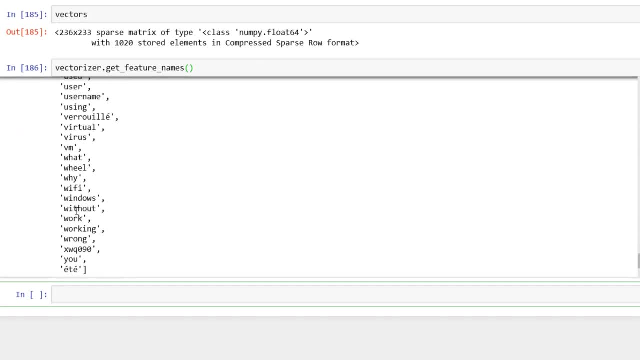 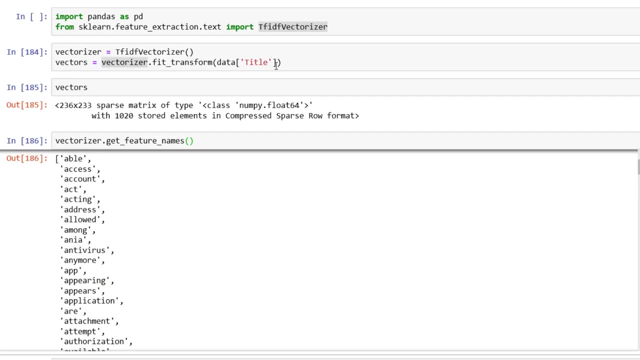 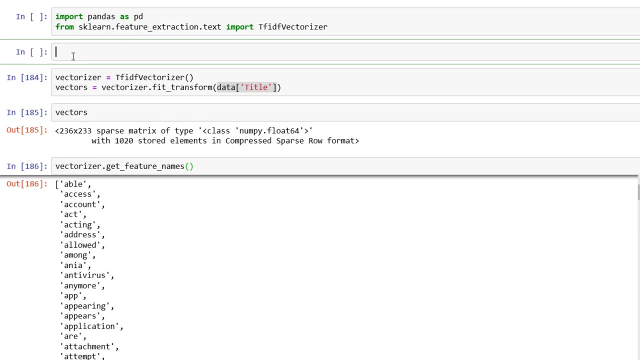 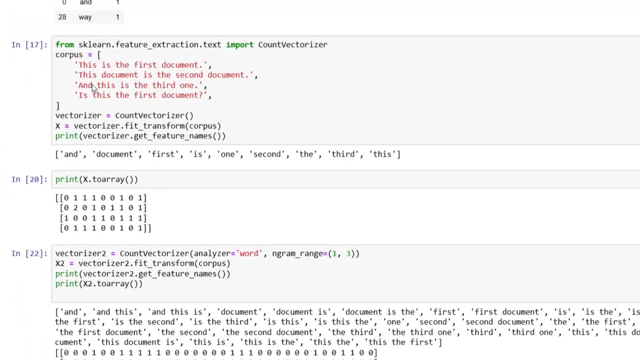 of all the words present in the complete corpus. so there are two more things in tf idf. one is the this data title. if i just show you a glimpse of this, it it needs the complete sentences, as you can see here. okay, so we have pre-processed the sentence earlier. right, we did it here, as you can. 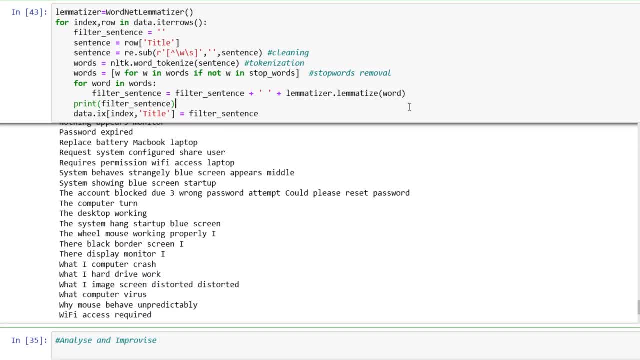 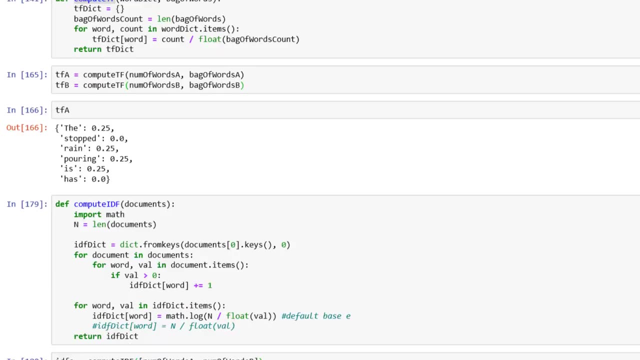 see. so what i have done is i have just, instead of getting the tokens of, instead of getting the tokens of sentences in the data frame, i just converted those tokens into the sentences again by joining them with the space. all right, so nothing much. you just want to give the complete sentences and it will automatically. 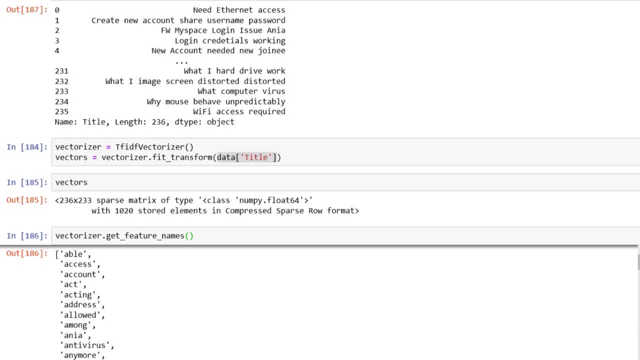 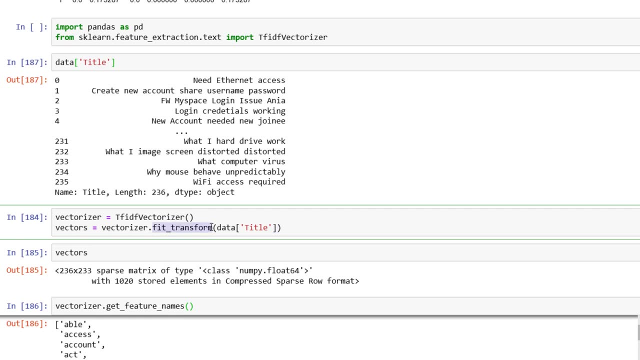 tokenize those, so you don't have to worry about this. and the second thing is this fit underscore transform. so you might want to know what is this fit underscore transform? so, basically, if you just do fit, it will create the list of all the words that are present in the data frame and then you 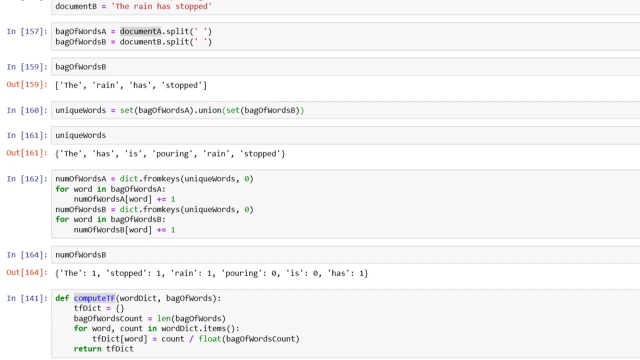 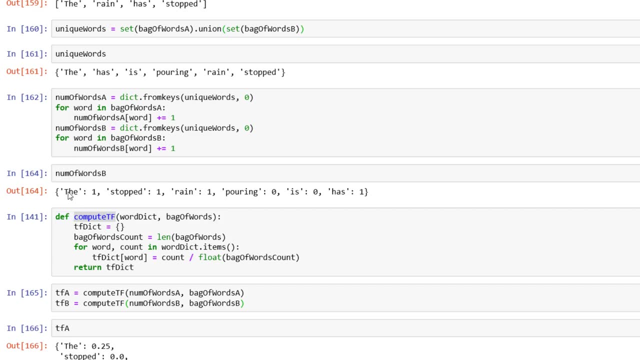 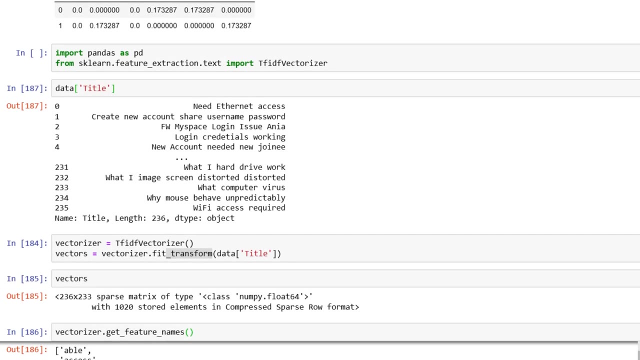 the dictionary, a dictionary like this that we have created here, okay, and then each dictionary, as you can see here, holds a position: the is having the zeroth position stopped is having the second position right, and once the dictionary is created, you will do the transform wherein transform your? 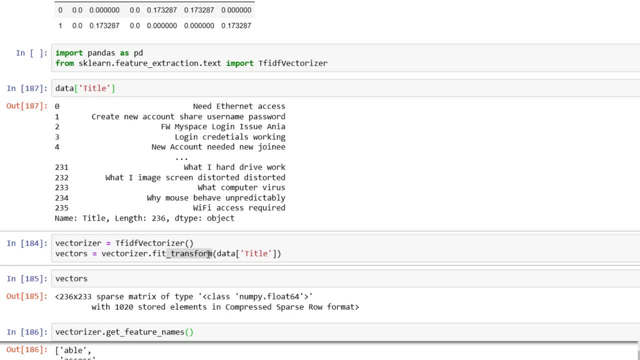 features will be created. your tf, idf values will be calculated. so if you do this thing on test data, right that you will be doing in the next video- we will be doing only transform in the test data, because we on we want to follow the same dictionary.